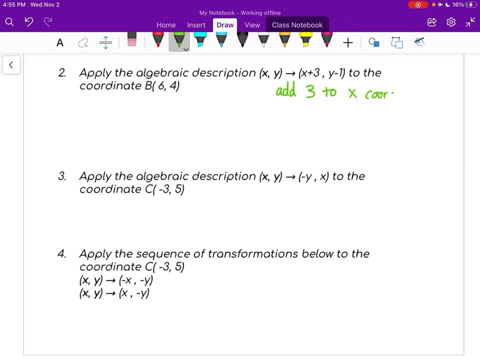 to our x coordinate. Y minus 1 means that we're subtracting 1 from our y coordinate. So if we started off with 6 and 4, we need to add 3 to the number 6.. So 6 plus 3 gives us 9.. 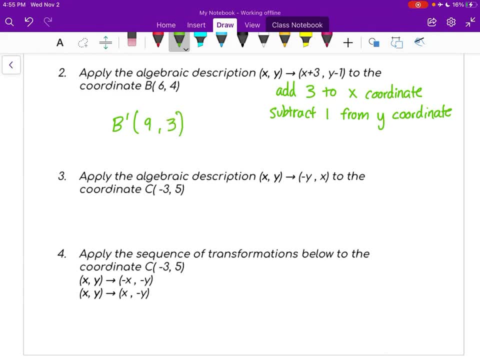 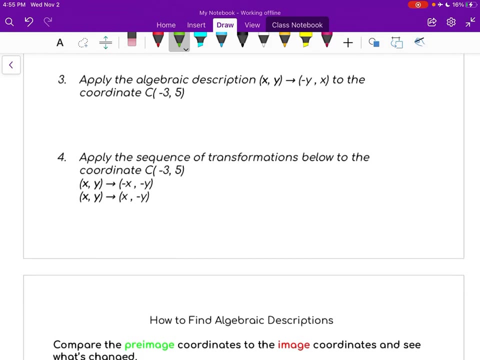 And 4 minus 1 gives us 3.. So this is the result of applying the rule x plus 3, y minus 1.. Let's move on to number 3. now For number 3, we need to apply the rule negative y, positive, x. 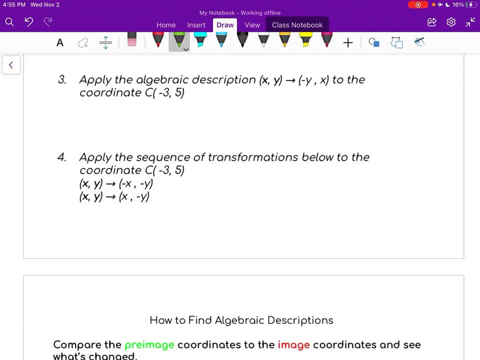 If you look carefully, what this means is that we've actually switched our x and our y coordinate. Not only that, but we've also multiplied the y coordinate by a negative. So let's do that. If I start off with c at negative 3, positive 5, switching the order of those two numbers would give me positive 5, negative 3.. 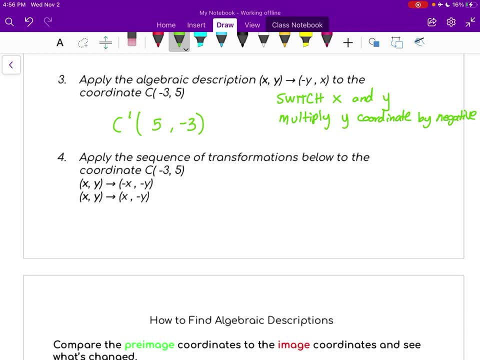 Now that I've switched the numbers around, I'm going to multiply the y coordinate 5 by a negative, which becomes negative 5.. So the result of this transformation is negative 5, negative 3.. And finally, what we're going to do is apply a sequence of transformations to point c as well. 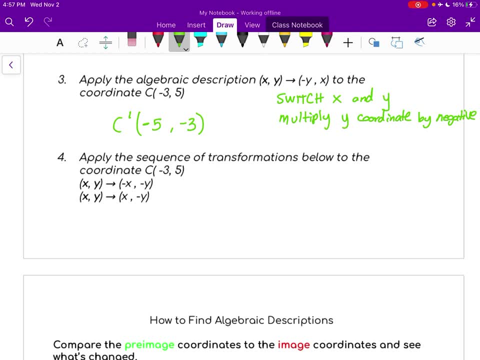 A sequence of transformations just means that we're doing more than one at the same time. So let's go one by one through each of these descriptions. Negative x, negative y means that we're multiplying both x and y by a negative. So if I take negative 3 and I multiply it by a negative, I get positive 3.. 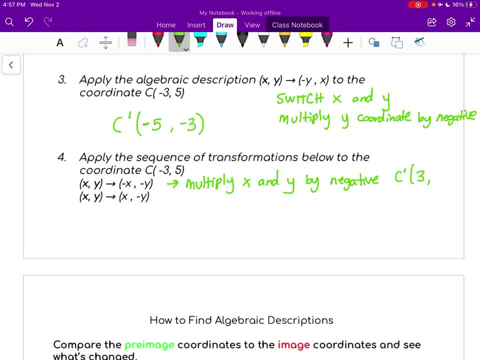 Because a negative times a negative is a positive, And if I take 5 and multiply that by a negative as well, I get negative 5.. However, now that I have 3, negative 5 as my result, I need to take that coordinate and I need to apply the second rule to it. 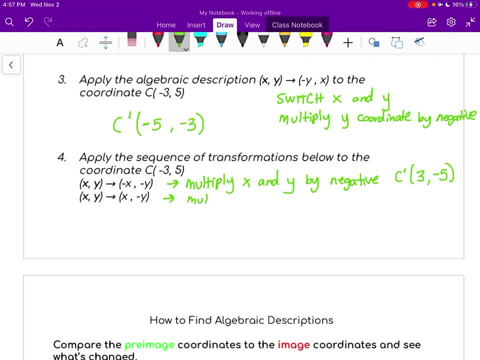 The second rule tells us that we just need to once again multiply the y coordinate by a negative. So instead of negative 5, we would have a positive 5.. So our final result is positive 3, positive 5.. Now that we know how to apply these rules, let's talk about finding them. 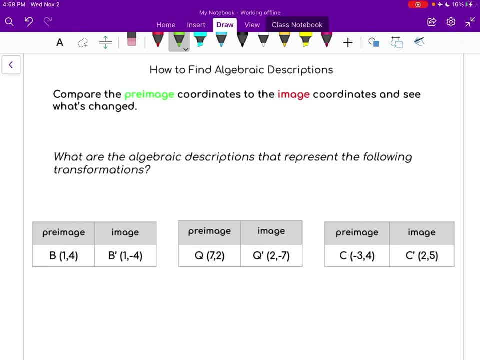 So think about what would happen if you weren't given these rules outright, or if you were just given a graph with nothing else. You can always determine the algebraic description for yourself if you just compare the preimage coordinates to the image coordinates and see what's changed there. 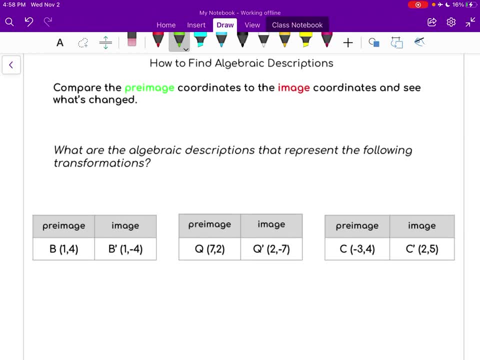 So let's do that with these three pairs. If I compare coordinate b, which is our x y, to coordinate b, prime, the only thing that changed here is that the y coordinate became negative, So that's exactly what we should write for this. 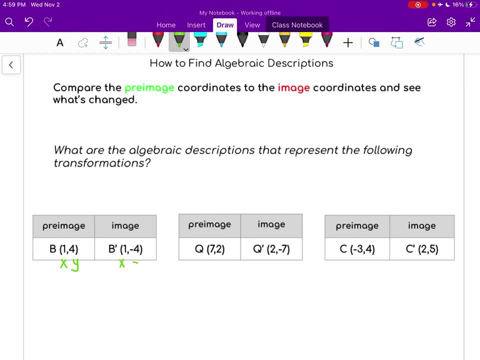 rule. We're going to keep x the same, but y is going to be negative now. So our algebraic description should look something like this: xy transforms into x negative y, And that's all there is to it. So let's do it with the second problem. If I compare q 7, 2, to q prime 2,, 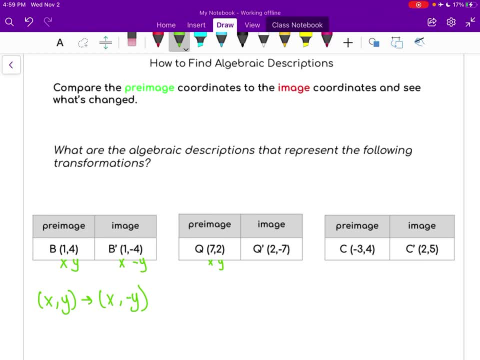 negative 7,. you'll notice that the order of the numbers has been switched around, So instead of being xy in that order, it now becomes yx. But that's not the problem. That's not the only thing that's changed. The 7 that we started with has now become: 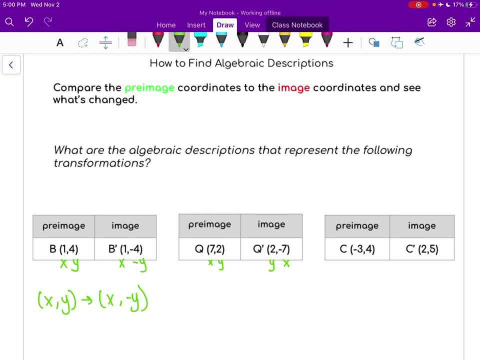 negative 7.. So the x coordinate is actually the one that became negative this time. This leads us to our rule, which says xy transforms into y negative x. Now let's look at c and c prime. c and c prime are a little more difficult because these are not. 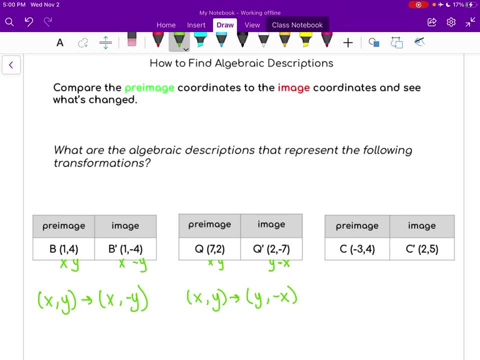 the same numbers that we're looking at. Something else is going on here, So we need to think about how we went from negative 3 all the way to positive 2.. And the only way for us to get there is if we add 5.. 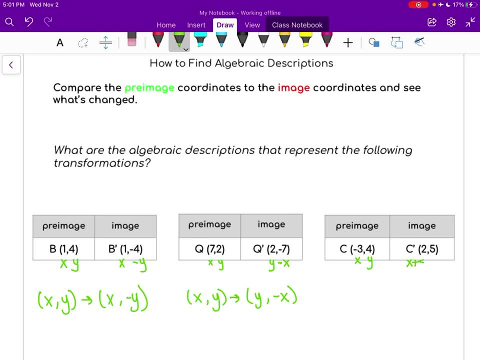 We can use the same reasoning if we look at how we went from 4 to 5.. To go from 4 to 5, we just have to add 1 to our y coordinate. So that's exactly what our rule becomes: xy transforms. 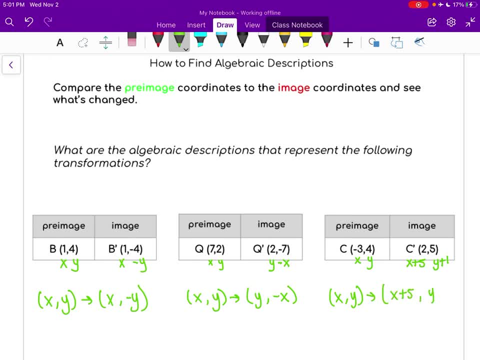 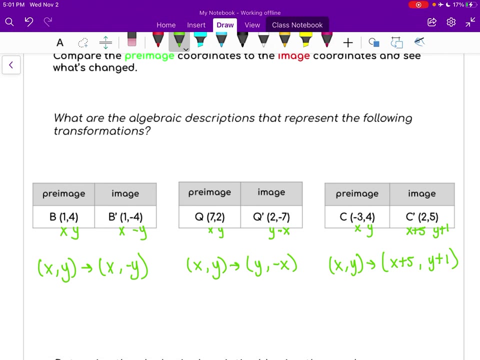 into x. So that's exactly what our rule becomes. xy transforms into x. So that's exactly what our rule becomes. xy transforms into x. Now let's take this a step further. If we look at these rules, we should be able to tell what type of 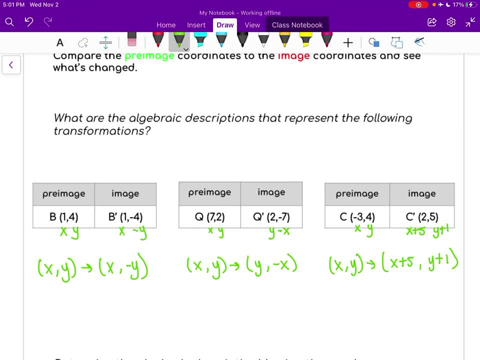 transformation is happening here, And you could do this one of two ways. You could just memorize each type of formula or you can actually graph these points To see what's happened on the graph Now. x negative y is actually the algebraic description for a reflection about the x-axis. 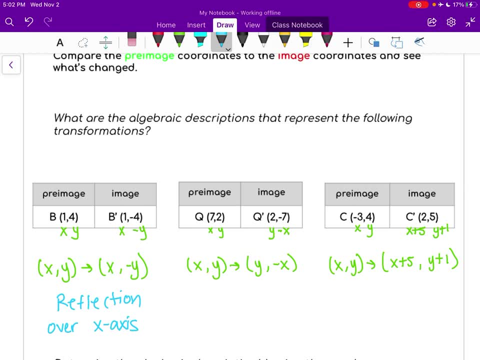 If we look at the algebraic description for q and q prime y negative x, This is a rotation. more specifically, it's a rotation 90 degrees clockwise. This is also the same formula that we would use if we're going 270 degrees counterclockwise. 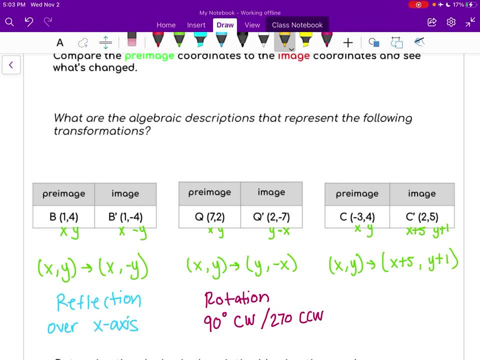 And finally, looking at c and c prime, since we're adding to x and y, that means that this is a translation: More specifically, x plus 5 means that we're going 5 units to the right and the y plus 1 means that we're moving 1 unit up.